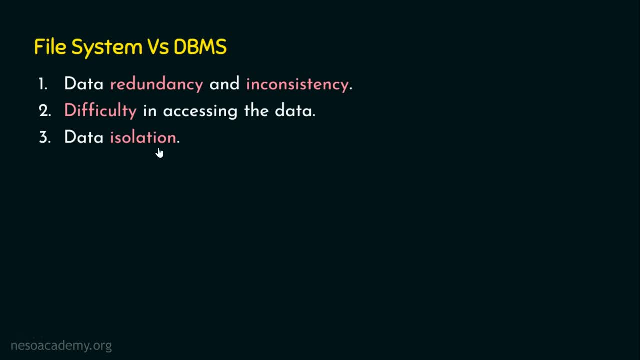 in accessing the data. Point number three: data isolation. Point number four: integrity problems. Point number five: atomicity problems. Point number six: concurrent access anomalies. And point number seven, security problems. I mean to say, these seven problems are there in file systems and that's why. 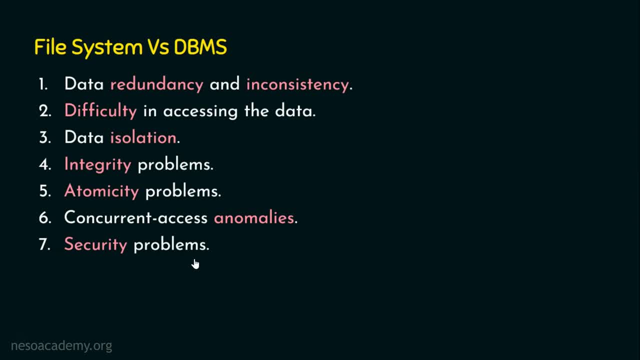 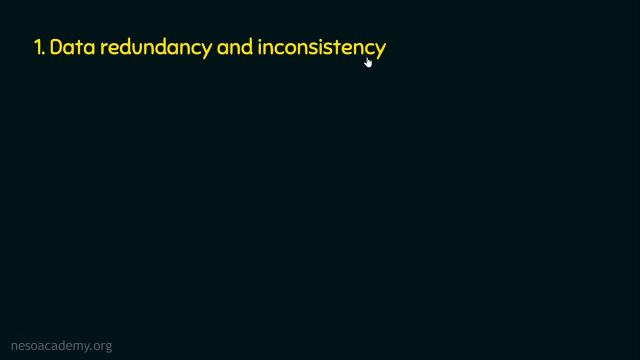 they are not suitable for organizations for efficient storing and retrieving purpose. Let's start with the first one: data redundancy and inconsistency. When we talk about software applications we know that software applications are developed by different programmers. Say, if we have a software program, that software is not the outcome of the effort of only one programmer. 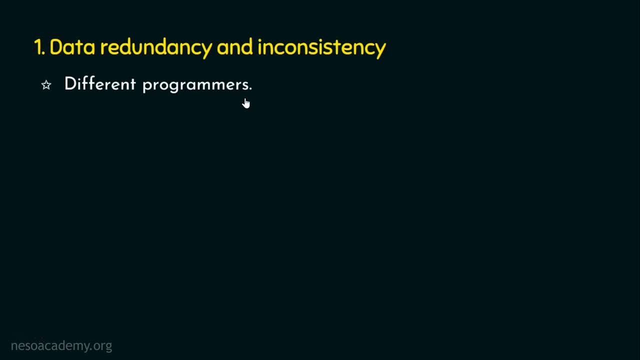 There are multiple programmers involved. When we have different programmers involved in creating a software program, So obviously we need to have a software program that is not the outcome of the effort. So obviously we need to have a software program that is not the outcome of the effort of only one programmer. 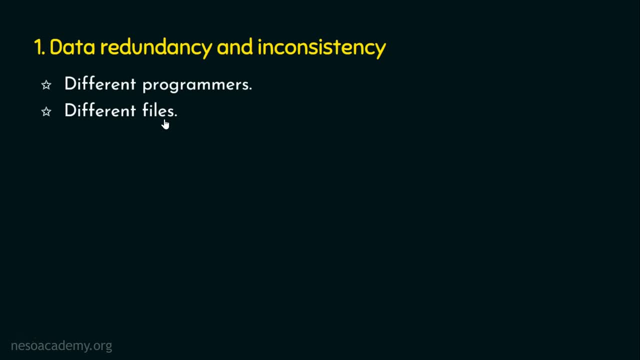 So obviously each programmer will choose different file for their own activities. When they go for obviously different files, obviously file structures are also going to be different. See: different programmers chooses different file systems. Obviously each file system will be differing in. 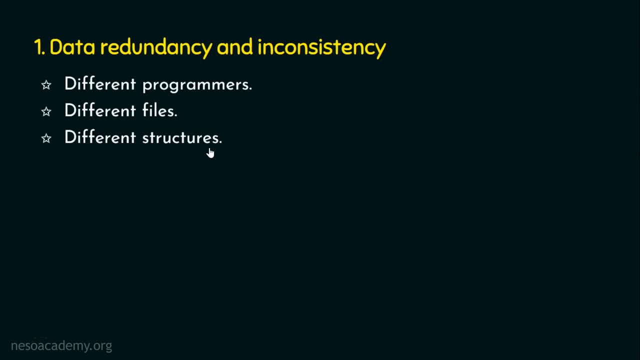 the structure and the way they organize the data. And at the same time, when we have different programmers involved in a software project, it may be using different programming languages. A software is generally a collective effort of multiple programmers, So each programmer has their own uniqueness. In that perspective, suppose if they store the data. 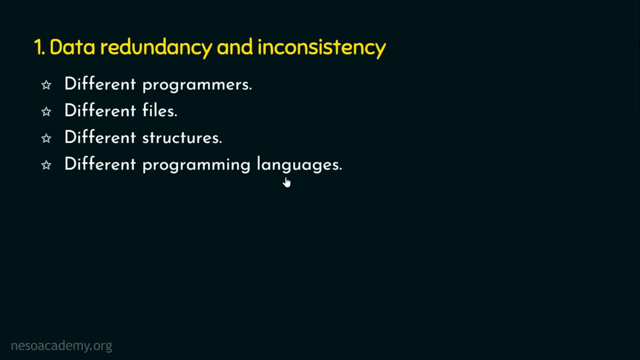 in different, different places. obviously, data is duplicated. So that is what I mean to say here- is, when we have duplication in the data, that duplication we call as redundancy. What is the disadvantage of having duplication or redundancy? Obviously, the storage will be. 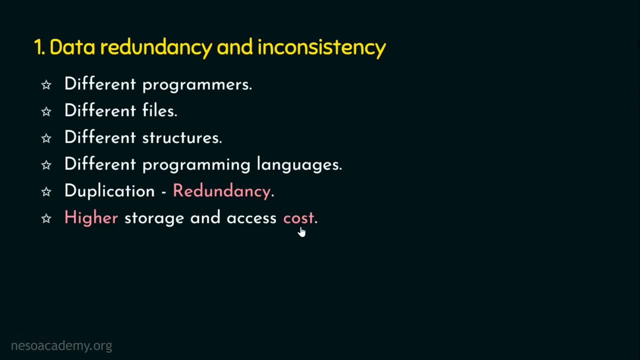 increased and the access cost is also increased. So when we have redundancy, this is a serious problem to address, because redundancy invites higher storage cost and access cost, And this is a problem mainly with the file systems, because each file can be stored in different locations as well. 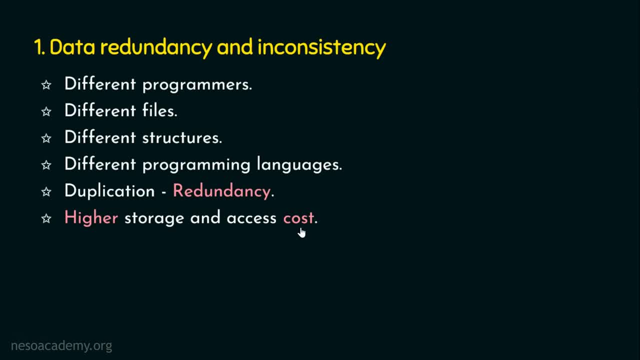 If we are working on Windows operating system, one file may be in C drive, another file may be in D drive. one file may be in one directory. another file may be existing in another directory which is not in the same drive. In such a situation, if there are duplicate records, 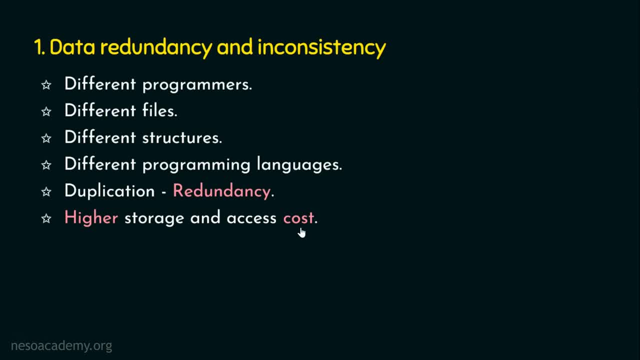 it's really difficult to find out which is the duplicate record. At the same time, when we want to access the data, it certainly invites a lot of access cost and the storage size is also getting increased Because of the redundancy. i will bring in a file to understand data redundancy and inconsistency now. 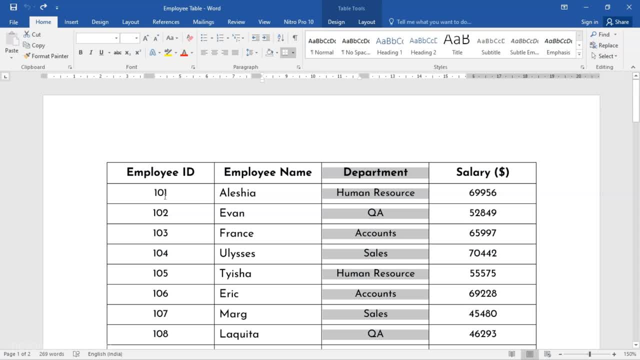 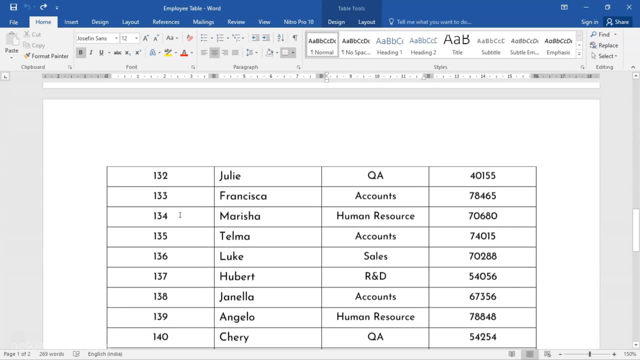 This is a table that I have created in Microsoft Word, where this table contains employee id, employee name, department and the salary of each employee. We can see different departments are there human resource, quality assurance, accounts, sales, etc. and I have listed few employees here- and the problem with maintaining this file system is that 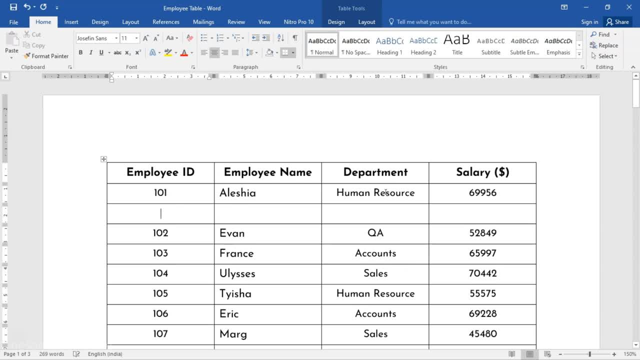 data redundancy. Say, if I insert a new row here, I'm just duplicating the first row, 101, Alicia, human resource and some salary. Now if you see here, this 101 is a duplicate record because we know already 101 exists. See file system is not able to identify that this is a duplicate record. We may be asking. 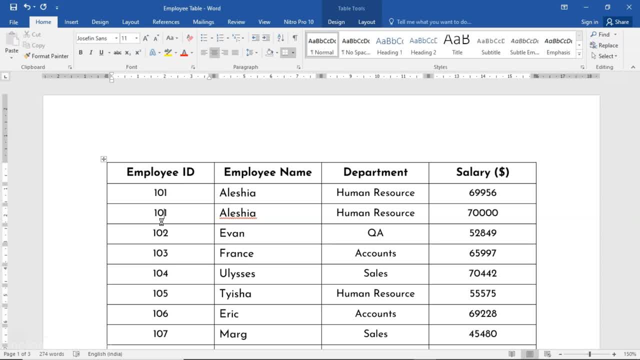 we can handle this situation well in Microsoft Excel by doing conditional formatting and formulas. of course we can do that, but think an organization wants to store and retrieve the data effectively. In such a case, if they go for file system, it's really difficult to access the data. 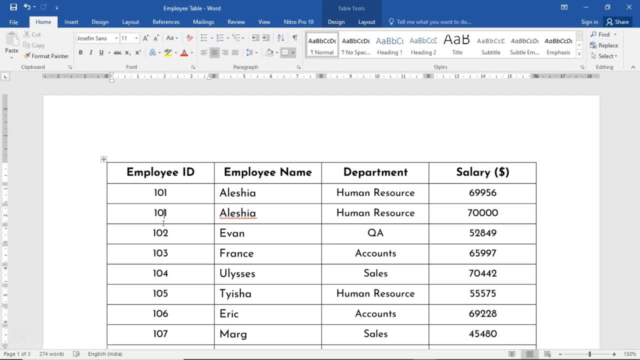 because handling redundancy is one of the biggest problems with file systems. At the same time, let's assume I am renaming the department human resource as simply HR. In this case, is it affecting the other places? No, We are making some change and we expect that change to be reflected in all associated places. 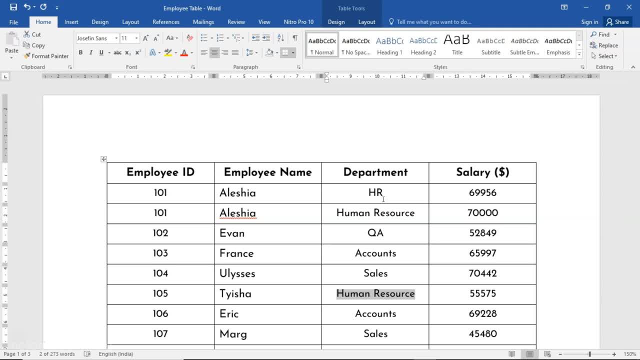 but unfortunately file system is not able to do this and this actually leads to inconsistency At the same time. let's assume one more situation. This file is located in C drive of my computer. I have copied the same file in D drive as well. I am copying the file to another location, just to. 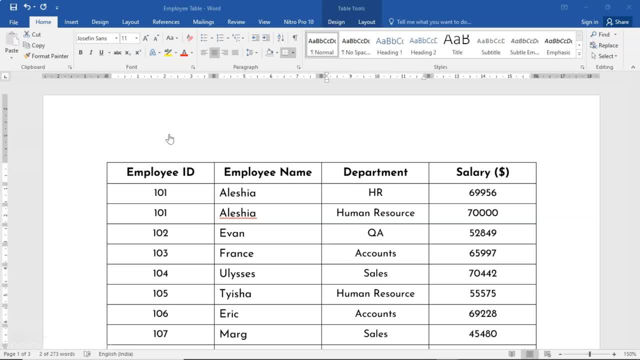 have a backup. I am copying the file to another location just to have a backup. Having a backup is always good because if one files get corrupted or lost we can still have another file. Let's assume I am making a change in the file that is existing in C drive. Will the 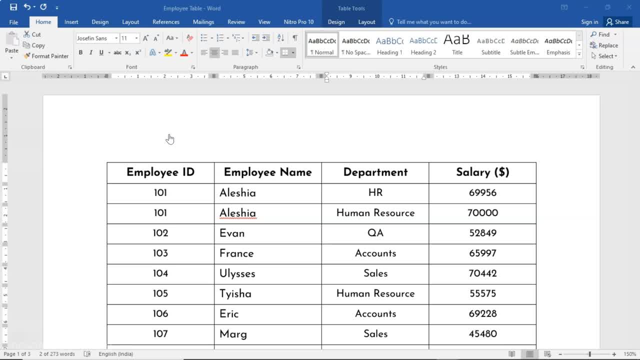 file present in D drive will automatically gets updated with the change that what we have done in the file that is present in C drive. No, This is also leading to inconsistency. Manually we need to go and update all the associated places if there is a change in the file system. but database systems are good in this perspective. 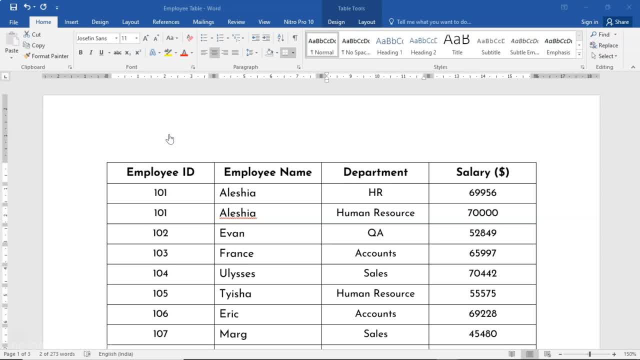 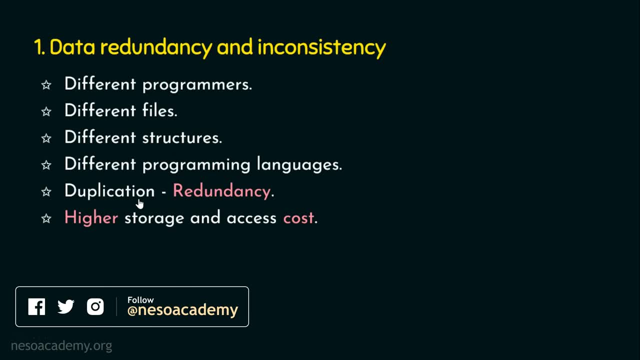 When you make a change in one place, it will automatically reflect the changes in all the associated places. That's the power of having DBMS. From this we understood that duplication- i mean redundancy- is a problem with file systems, and databases can handle this well, and also file. 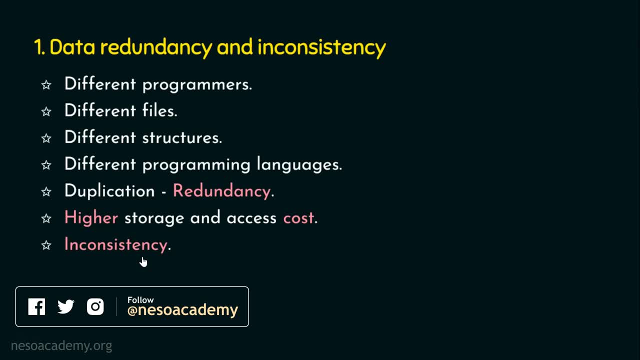 systems has inconsistency, which can also be handled well in database systems. how database system handles well. don't worry about this now. when the course progresses we will be able to understand all the stuff right now into anautocul in database solutions stuff completely. So we are done with the first point: data redundancy and inconsistency. Let's now 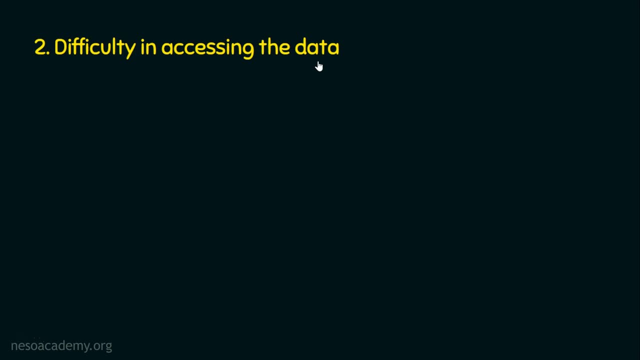 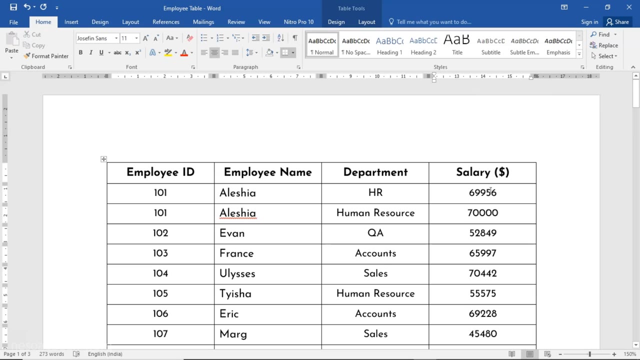 move on to the second point: difficulty in accessing the data. Let's take the same file, The example, what we are seeing. I am asking you to retrieve all the employee names who draw salary greater than 50,000.. In that case, retrieving the data from a file system is really difficult, As already. 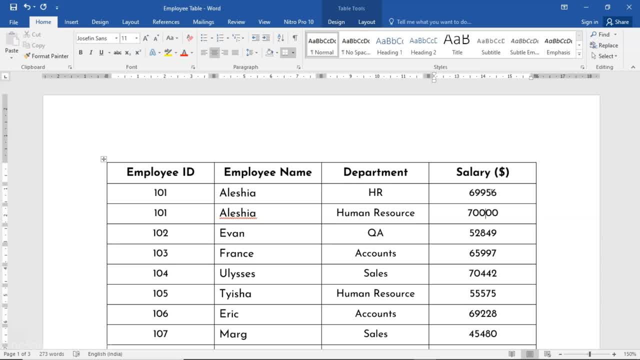 mentioned, if you work with a file system, if you apply filters or conditional formatting, you can retrieve it. But think when there is an application and that application requires the data from your file. In that case it's really difficult. Only thing is you need to manually go and check, is it? 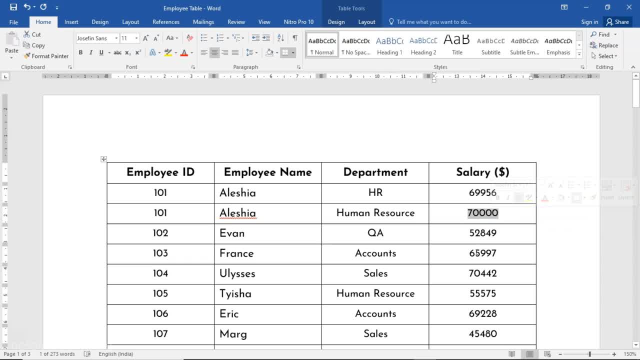 greater than 50,000? Yes, Is it greater than 50,000? Yes, We have to manually retrieve all the records and in this case, here, this is not greater than $50,000.. So we need to remove this or we need. 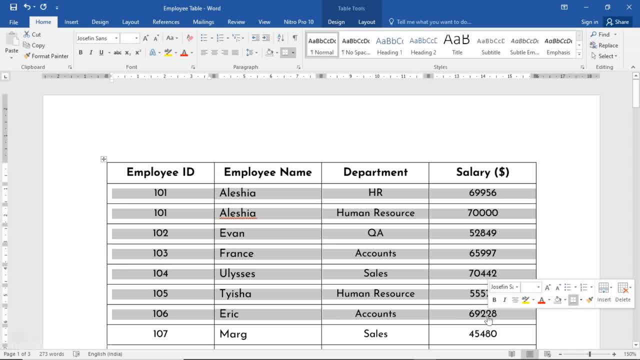 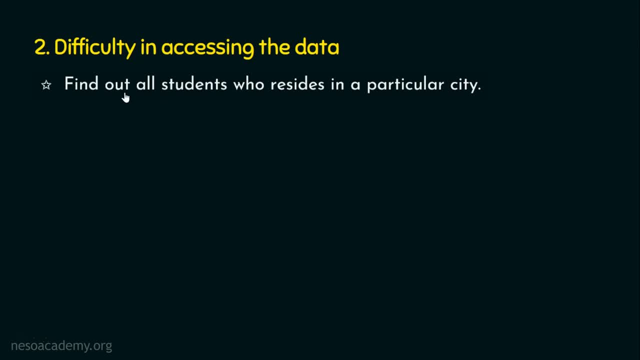 to copy all this. So it involves a lot of manual effort and that's why I told you file systems have difficulty in accessing the data. Let's take two examples. Just imagine I have given a file which contains all student information in a table and I'm asking you to find out all students who resides in a. 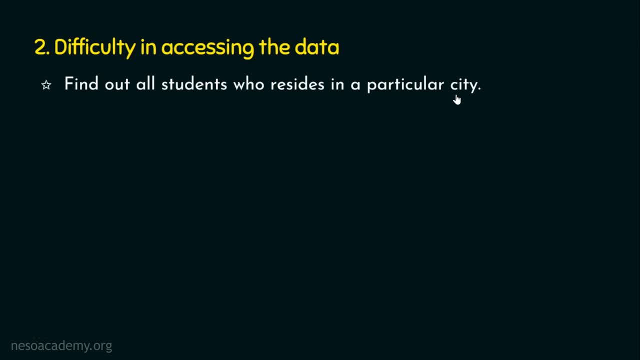 particular city. As already mentioned, we need to manually do it in case that city has multiple names and that refers to the same city again. In that perspective it really invites a lot of inconvenience. So file system is really having difficulty in accessing the data And I'm asking: 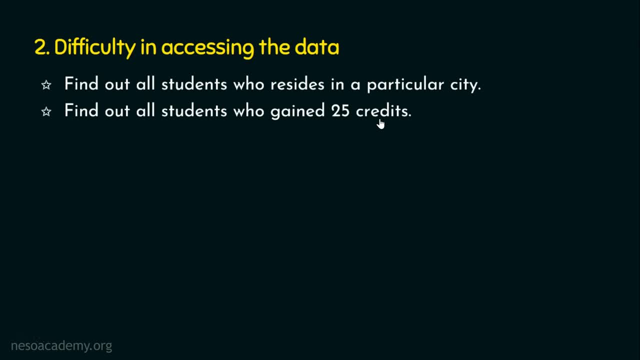 you to find out all the students who gained 25 credits. In such a case, manual intervention is really required And see the real difficulty again. Now I am asking you to list both. I mean all the students who resides in a particular city And also they should have gained 25 credits in. 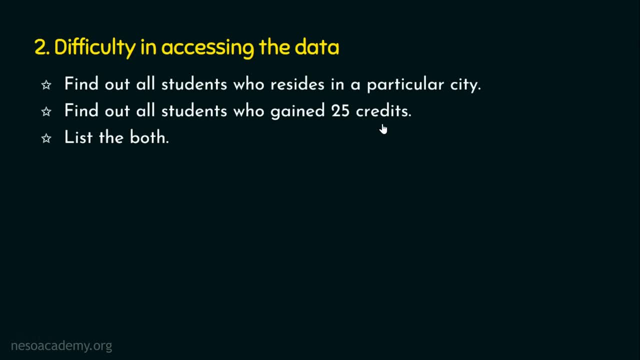 this case, file system is really difficult in accessing the data, But database systems are very easy. when we supply the queryies with the condition they should belong to this city and they should have gained 25 credits, It's really easy in DBMS to access or retrieve the records as per our convenience and conditions From this. 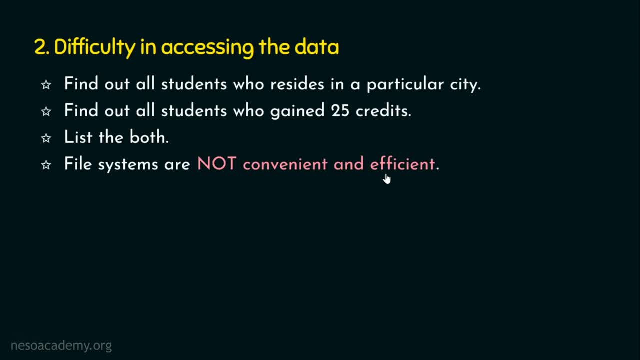 we understood that file systems are not convenient and efficient, whereas database systems are. So obviously, when we want to have easy access, easy retrieval of data, then a more responsive data retrieval system is needed, which file systems cannot offer. Fortunately, DBMS can do this easily. 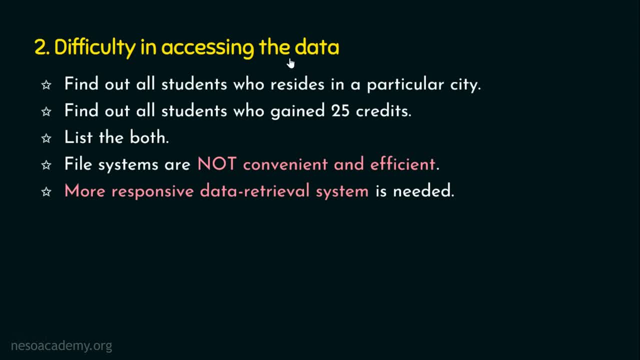 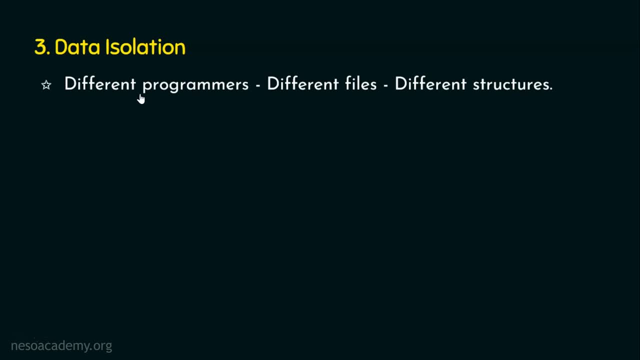 We are done with the second point: difficulty in accessing the data. Let's now move on to the third point: data isolation. What do we mean by this? We know software programs are the efforts of different programmers where they use different files, where each file uses different file structures. 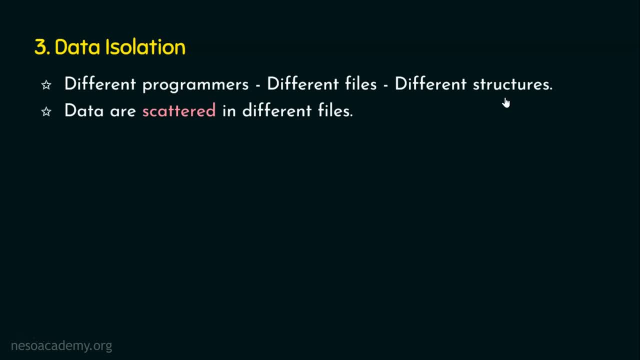 and obviously they may store the data in different locations as well. So obviously the data are scattered in different files in file systems. In such a case, isolating the real data that we require is a problem, Because our files may be in different locations, and that's why data isolation is really difficult. 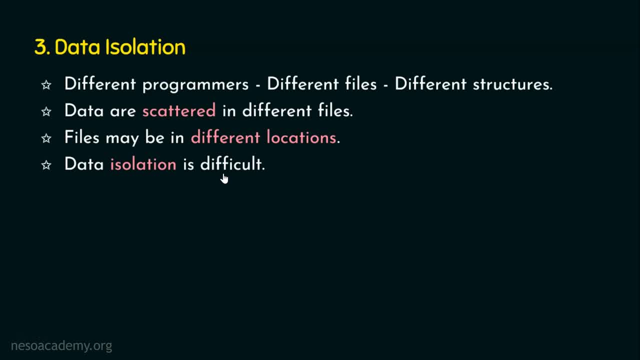 with file systems, But in DBMS all the records are going to be stored in a central place, which is the database, and that's why, whenever any change is made in one place, all the associated places gets updated automatically. At the same time, data can be easily isolated because all the data are in. 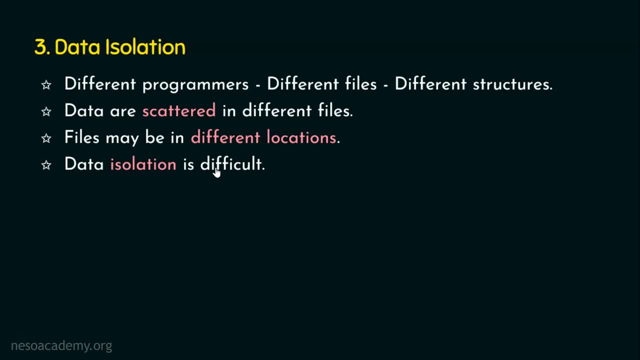 one database And you may be asking how come, if that database fails, what we should do? All data will be gone right, No problem. we can take backups periodically and we can synchronize the backup with the up-to-date data. So we are done with the third point, the data isolation. Let's now move on. 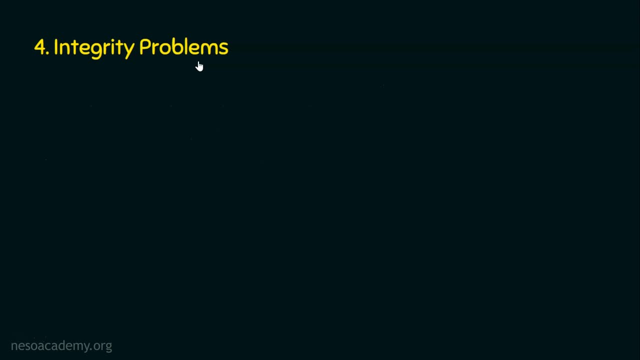 to the fourth one, the integrity problems. What do we mean by integrity problems? Suppose I want to enforce some constraints or conditions to my data, which is actually stored in the file system. Let me bring an example file. We know all employees will have salary, but here I am updating Alicia's. 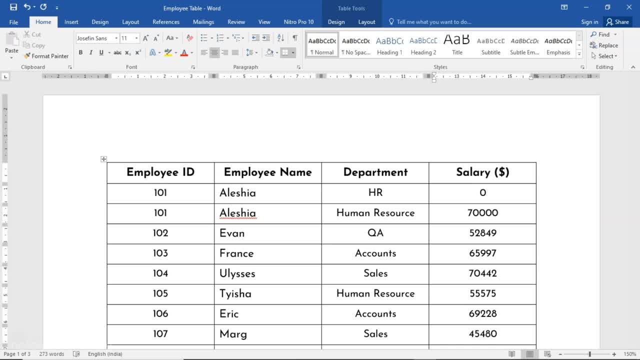 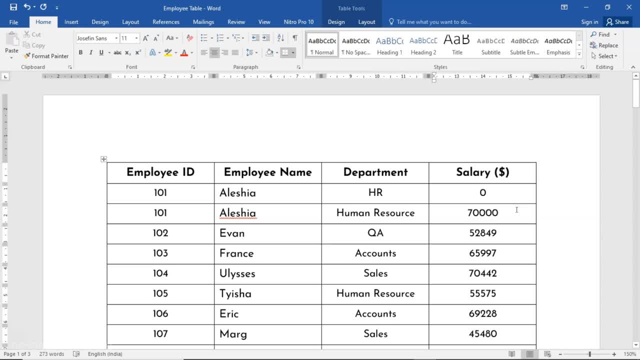 Because there is no way in this file system to enforce some conditions that the salary value should not be zero. So that's one of the biggest problems with file system. So when we want to enforce some conditions then definitely it is not possible with this file system. To some extent we 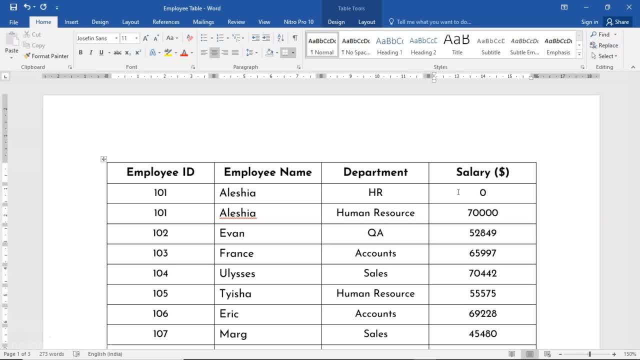 can handle this in Microsoft Excel. But again, as I mentioned, this file system cannot be a complete back-end, Because if we want to enforce some conditions, then we have to go through some constraints, Because there are several drawbacks and we are dealing all the drawbacks one by one. 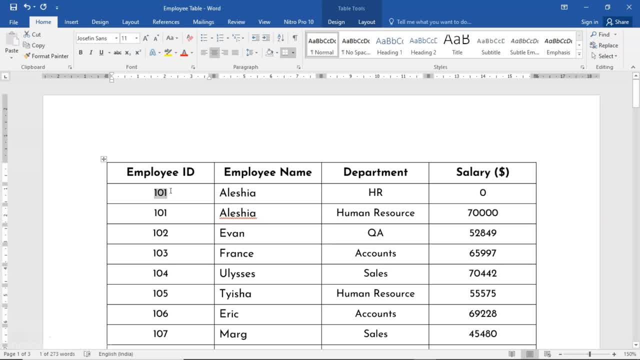 At the same time, if the employee ID is purely a number type and when I start giving a random text, it's accepting because no constraints can be enforced here. So this is also one of the problems with the file systems. So, coming to the integrity problems, we cannot enforce consistency constraints. 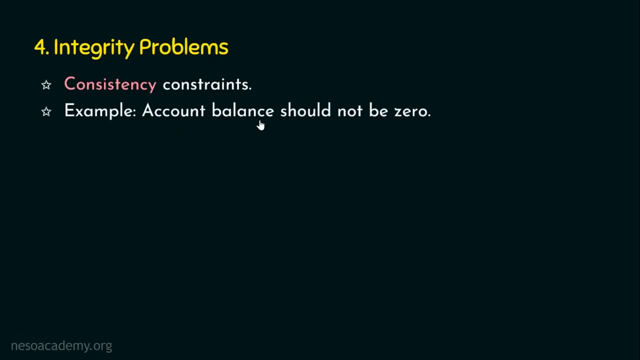 into the files. Example: the account balance in a banking database should not be zero. If this is maintained in a file system, definitely it's really difficult. But when it is a database system, when we enforce a condition that account balance should not be zero whenever, 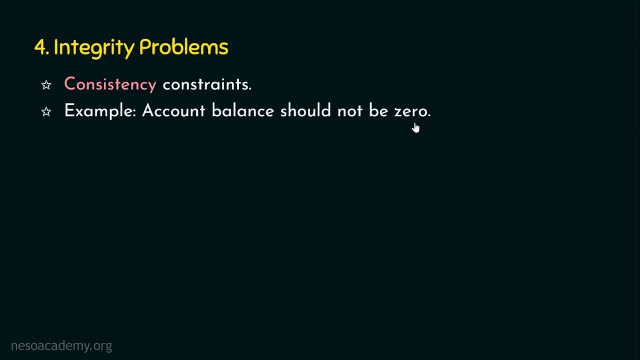 any update or insert is carried out on that particular row, and if the condition is not satisfied, then that activity will not be permitted in databases. See how powerful databases are. Of course, we can easily enforce these constraints or conditions in a software code. So it's really. 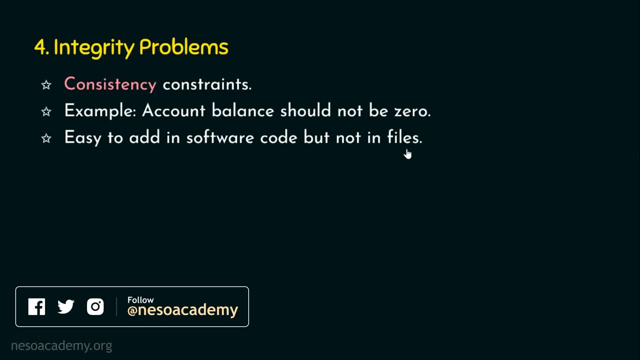 easy to add the conditions in software code but not in the files, And that's what we have seen just now. Think you have enforced some constraints and suddenly we want to enforce some constraints Again. this is also a problem with the file systems, But in database management systems. 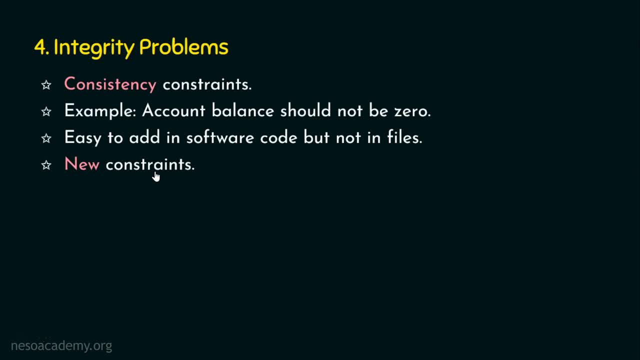 anytime, whatever constraints we want to enforce. we can do that because databases are really a savior for all these problems And we have one more biggest integrity problem with file system, which is this problem. The integrity problem is compounded when the constraints involve several. 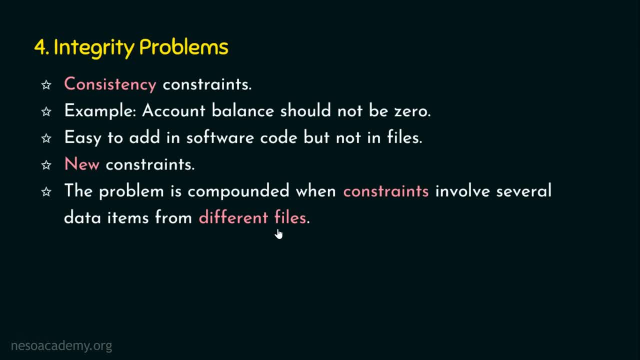 data items from different files. Imagine our data is scattered or stored in different places- different files. Imagine our data is scattered or stored in different places- different files. In that case, enforcing some constraints when it involves several data items will be really a tough. 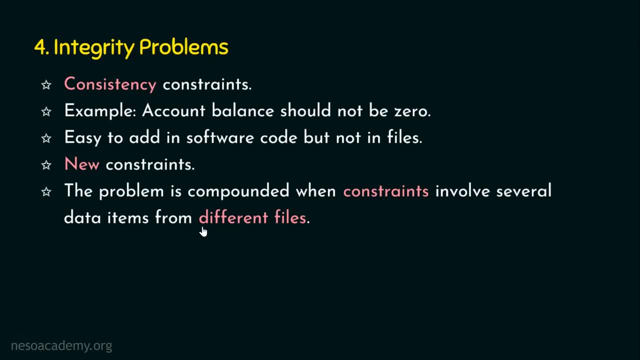 task. But this will not be the case in database management system, because all the required data will be in our database in one place. So we are done with the fourth problem, the integrity problems. Let's now move on to the fifth point, that is, the atomicity problems. File systems are 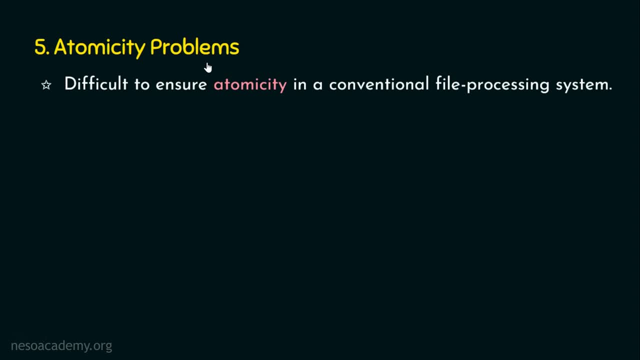 really suffering from atomicity problems. What do we mean by this? It's really difficult to ensure atomicity in a conventional file processing system. What do we mean by this? Don't worry, I am going to explain that now. See any system, whether it is a hardware system or software system. 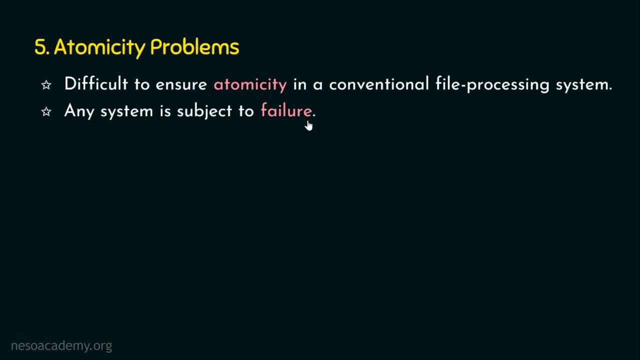 any system is prone to failures is subject to failure, isn't it? When a failure has happened, it is an expectation from that system to recover from failures. Of course, backup will be really helpful in doing this. So, obviously, restoration of data is a very, very essential thing when the 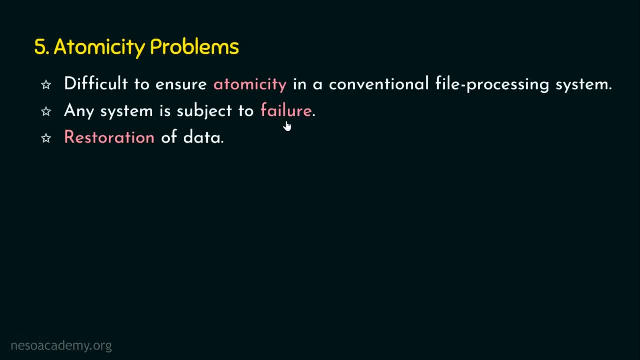 system encounters failure. So let's now move on to the fifth point, that is, the atomicity problems. Now, when we have a backup, we can easily restore the data. I am not talking about the problem of backup here. I am talking about atomicity problems. What do we mean by this? 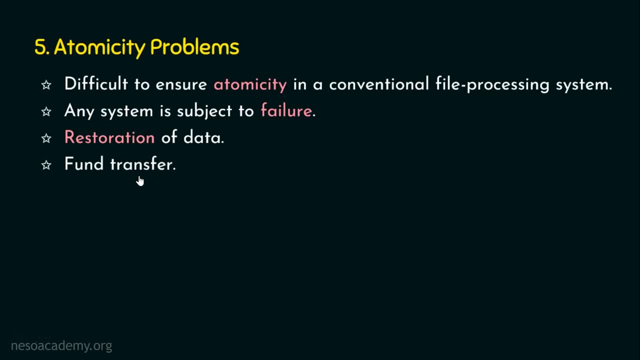 See the example, then you will be able to understand this. Let's say I am doing a fund transfer and I am going to enforce a condition that that transaction should be atomic. It means the transaction should fully complete or none. I know things will be unclear When we 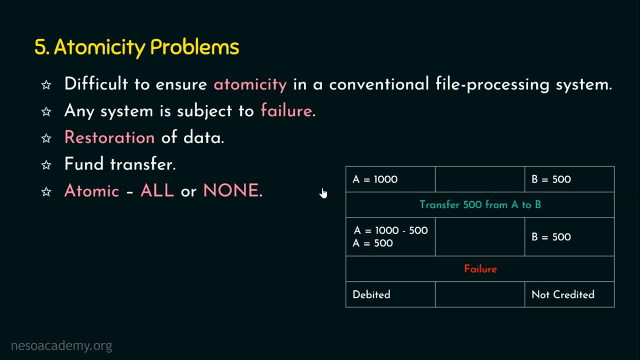 see an example, then it will be easy for you to understand. Let's bring in a table here. Let's assume I am going to do a fund transfer from A's account to B's account, So this is what the example that I was talking about Let's assume before the transaction is started. A is having the. 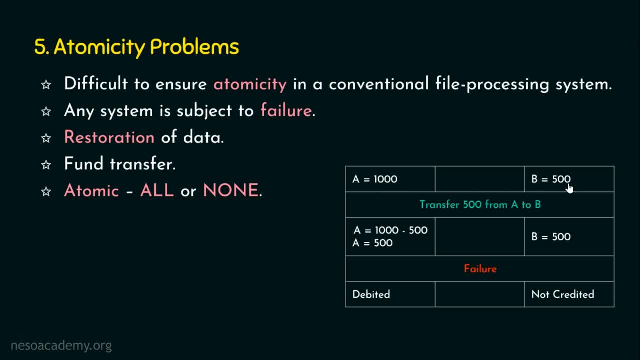 account balance of $1,000 and B is actually having the account balance of $500. And let's assume the transfer operation is carried out from A's account. I mean transfer of $500 from A to B. It means from A I am withdrawing $500 and the new balance for A will be only $500. 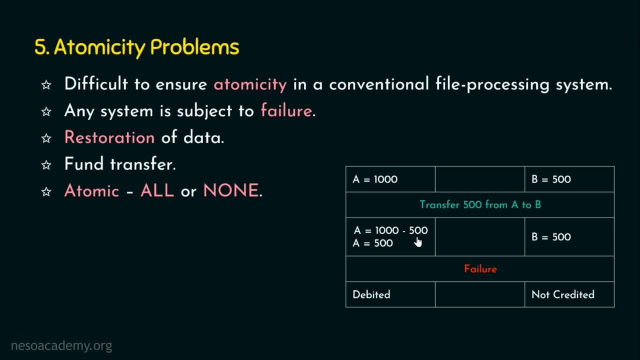 Because this $500 is debited to A's account and it is expected to be credited to B's account, isn't it? So at this stage, A is having a new balance of $500.. Remember, the debit operation is completed, but still the credit operation is not completed After debit is completed. 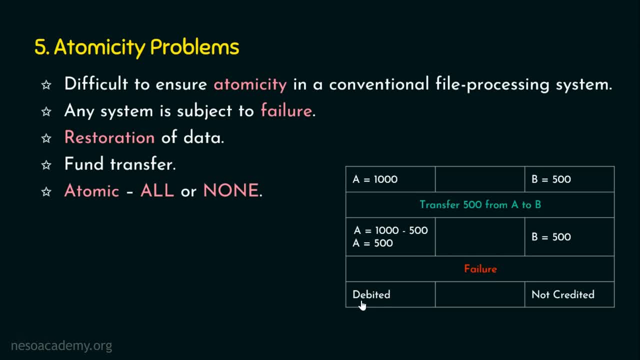 let's assume the system has undergone a failure. In that case the value is actually debited and A is ended up with only $500 and if you note, here the value is not credited to B's account. B is also with $500. only When a system is accepted, if A is $500 and B is $1,000, it means amount is. 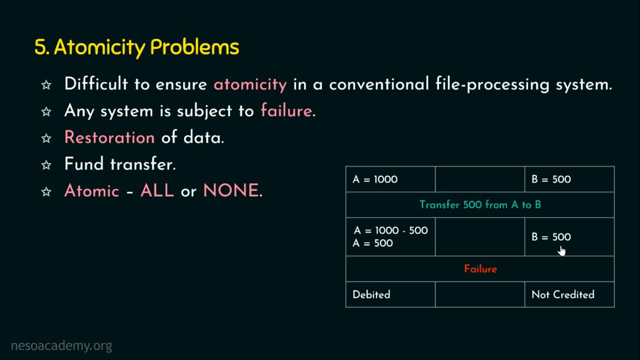 debited to A's account and credited to B's account. That's perfect. Otherwise, the money should have not been debited to A's account, so that consistency is maintained. See, this is a real problem when we deal about transactions, when we use files as a backend. So what condition I am enforcing is: 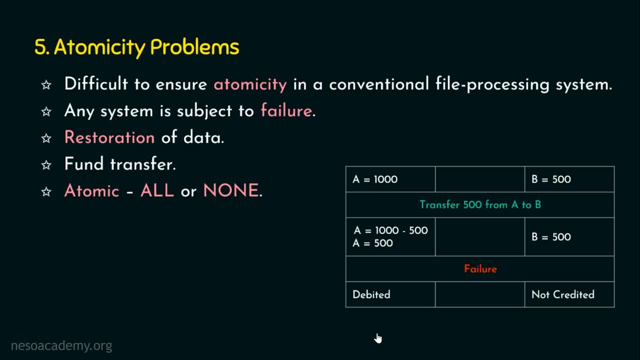 if a transaction is started, it should complete till the last. When the source account is debited, the destination account should get credited till the last. So I am enforcing a condition: if a transaction is started, it should complete all, otherwise none Say if a failure is happened. 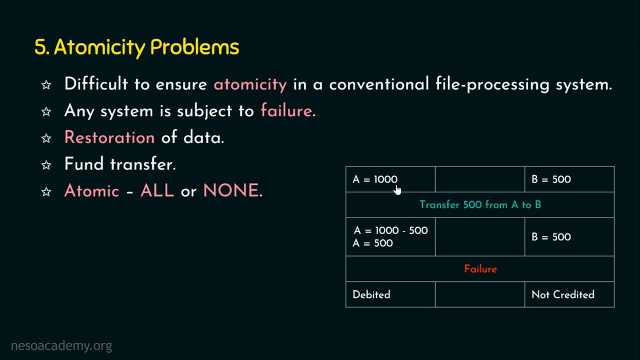 here, then the transaction should be revoked to the previous stage, with A is $1,000 and B is $500. even there are some statements executed and if there is a failure, so the system should identify the failure and it should revoke it to the original place, like A is $1,000 and B is $500. 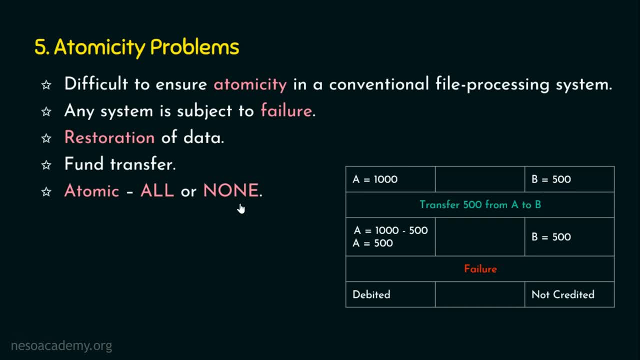 we are achieving All or none right. If all, then good, If none, that is also good. Partial execution obviously is not good in this stage and that's why we want to enforce atomicity constraints to this and that's why I am telling you: file system has a lot of atomicity problems. 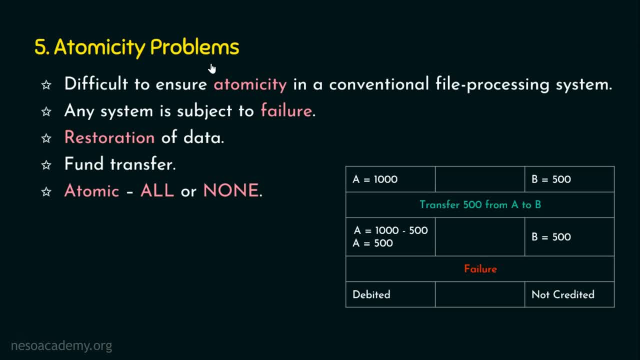 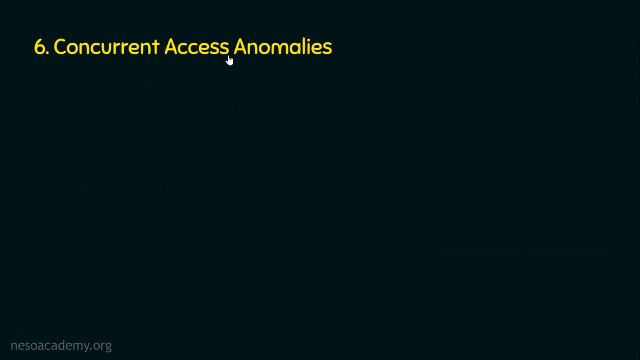 whereas DBMS is very good in this perspective. So we are done with the fifth problem, the atomicity problems. Let's now move on to the sixth point, which is concurrent access anomalies. Is concurrency good or bad? When multiple people work at the same time, it's always good, We know. 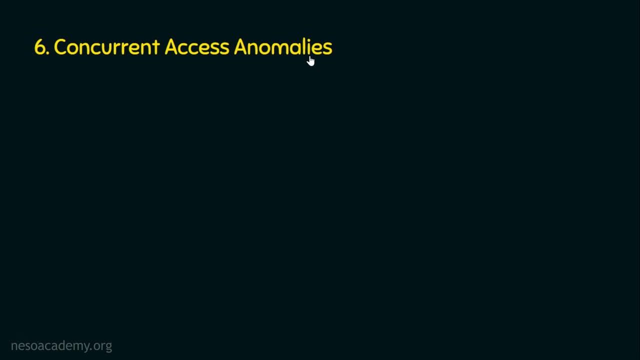 databases store all the data in one place, isn't it? Let's assume if one person is accessing the database, another person is refrained from getting the access because already one person is accessing the database. it's not good, right? Let's say we are accessing googlecom. See multiple people. 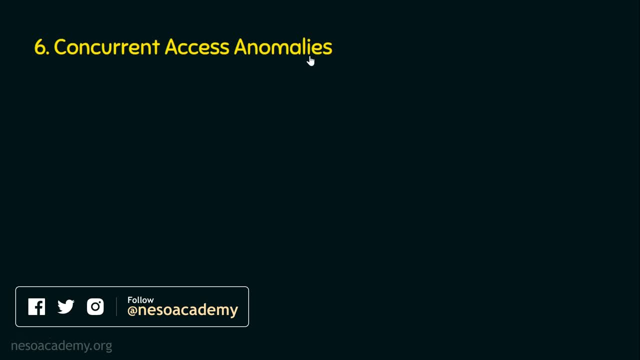 from multiple different locations are accessing the database, So we are not good at this. So concurrent access is always good, but there are some serious problem with concurrent access, and that, too, when they are accessing the same data. Let's see that now. So concurrency is. 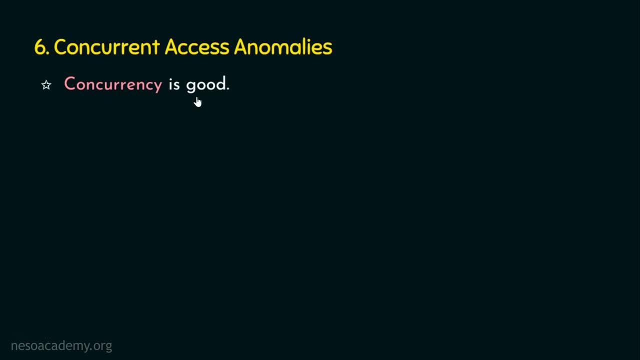 always good because multiple people can access the resource at the same time, but it may lead to inconsistency which we need to address How? Let me take a real-time example. Let's take there is a common balance to the department, which is one thousand dollars. So this department is 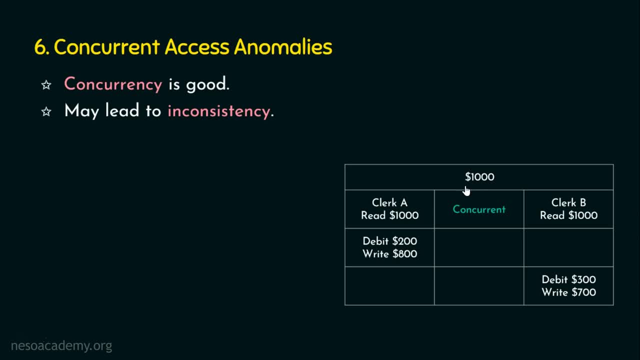 an account balance of one thousand. Let's assume there are two clerks. clerk A and clerk B can access this shared data item. Let's assume clerk A wants to withdraw some money. At the same time, clerk B also wants to withdraw some money. Let's assume the situation that both are doing this at. 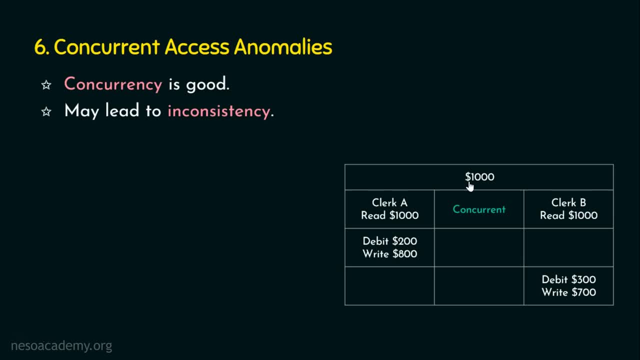 the same time. When clerk A reads the shared data item, the account balance of the department, he sees it as one thousand dollars. Same value only. clerk B is also going to see, because this is a concurrent access, So let's assume that both of them are doing this at the same time. 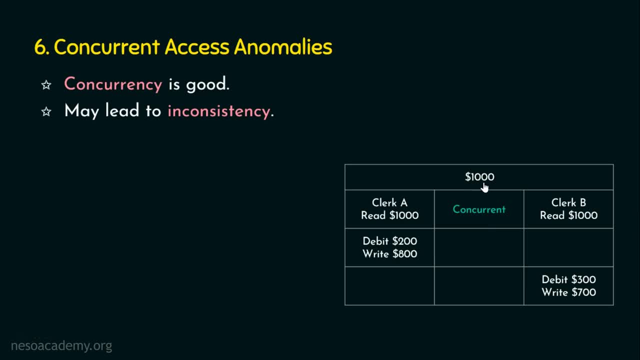 Both clerk A and B are accessing this shared resource, the common data, at the same time. After reading, let's assume clerk A is debiting two hundred dollars and he is writing a new value as eight hundred dollars, and this is correct only because one thousand dollars is the actual value. 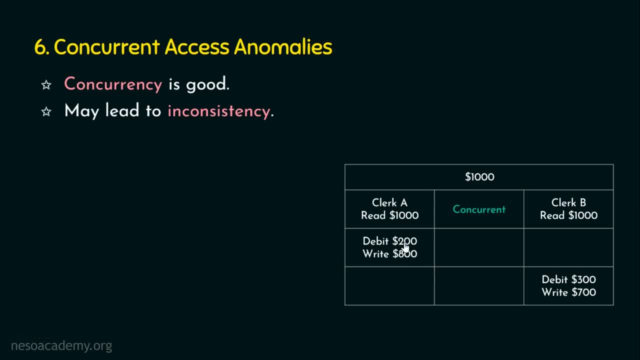 what he has read and he debited 200 to the account. and finally he is writing a new value, eight hundred dollars, which is perfectly fine. After A completes its execution, A has written a new value eight hundred and he has left the place B after he has read the value one thousand. after some time. now he is debiting three hundred to the. 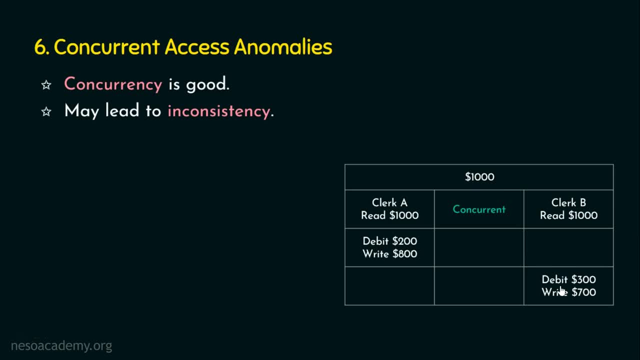 account. It means he has read one thousand, which is a wrong read, actually, because a new update was already carried out, But B is not aware of this. B assumes that the account has one thousand dollars as the balance, which is this, and he writes a new balance after debiting three hundred. The new. 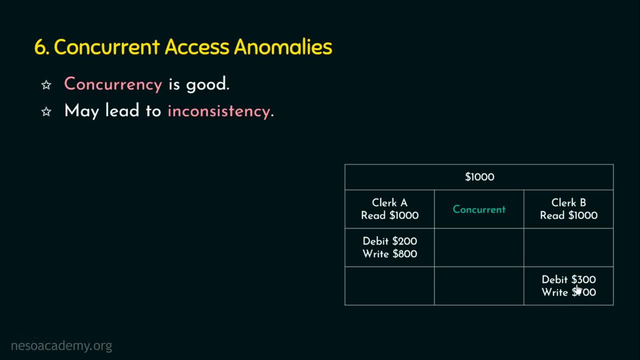 balance is what? Seven hundred according to B, And if B writes this as the final value to the common balance of the account- B is not aware of this. B assumes that the account has one thousand dollars as the or the common data, then this is a problematic one, because the new balance 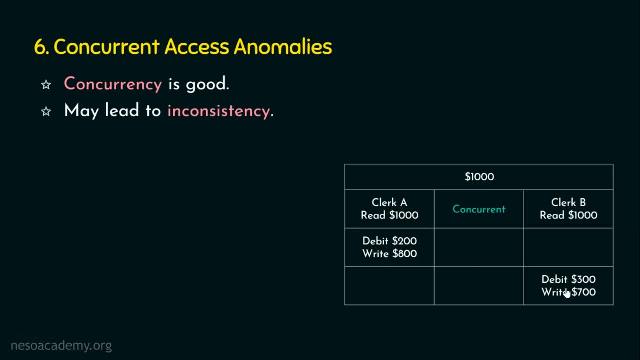 is 500 only. A has already debited 200 and B is debiting 300. obviously, 200 plus 300 is 500 and the new balance should be what? 500 only. but see what is the final value that is written by B: it's 700, which is definitely incorrect, and that's. 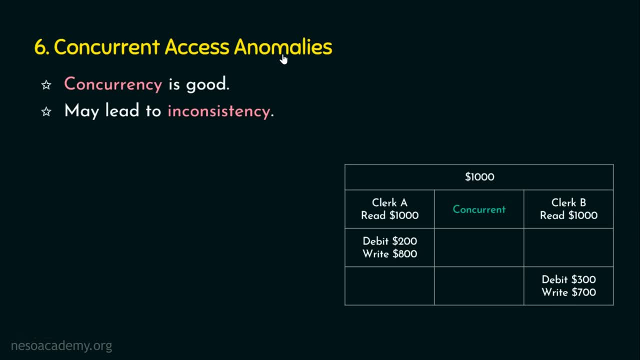 why I told you concurrent access. anomalies are there in file systems, but databases are really good in this perspective. even if multiple people access the resource at the same time, databases are good in handling this. I will also give you one more example. let's assume there is a file in a shared 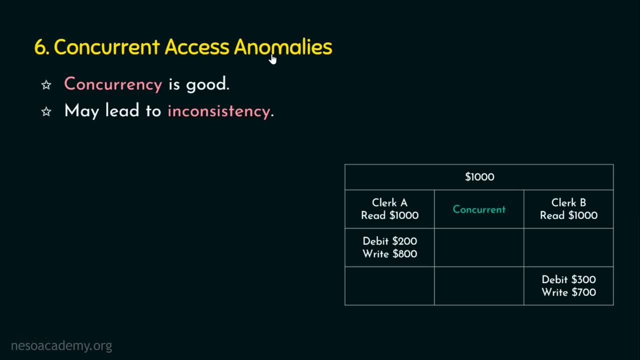 directory. what happens when two people open the file at the same time? the first person, when he opens, he gets both read and write permission on that file right in. the second person who opens the same file which is in the same location because it's a shared location, then obviously he gets the file with the read. 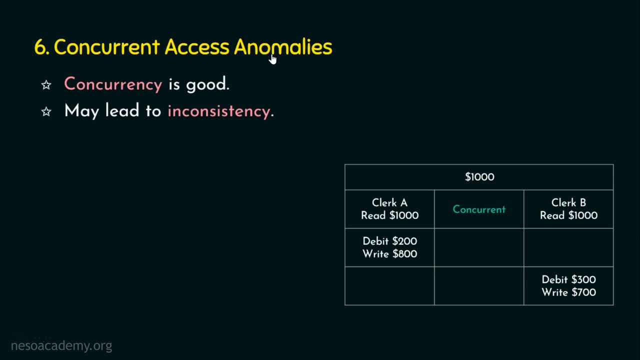 only permission, permission not with the right permission, because it leads to inconsistency when concurrent access is there in a file system, isn't it so? file systems are not recommended when we are going for concurrent access because files have a lot of anomalies. when we deal with concurrent access, we are done. 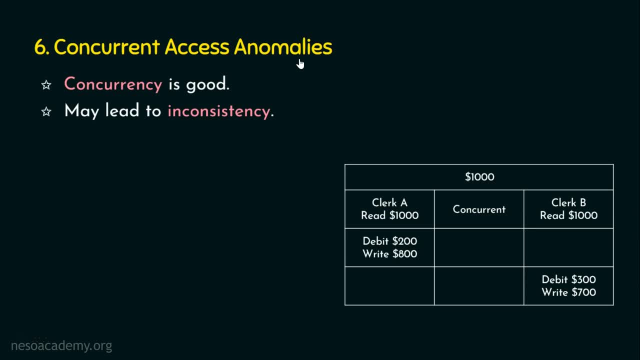 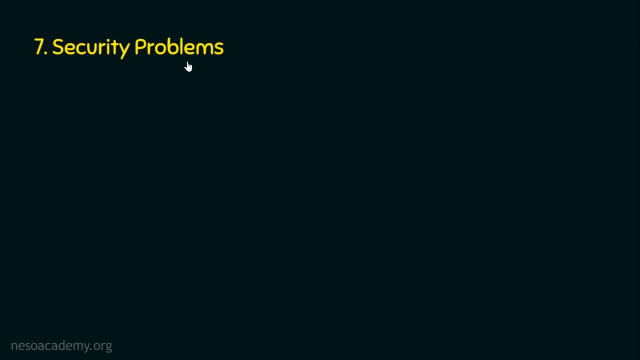 with the sixth point, the concurrent access anomalies in file system. let's now move on to the last one, the security problems. and we know security is important for anything, and we know databases or file systems, both are going to deal with the data. think about: the data is a confidential data, so 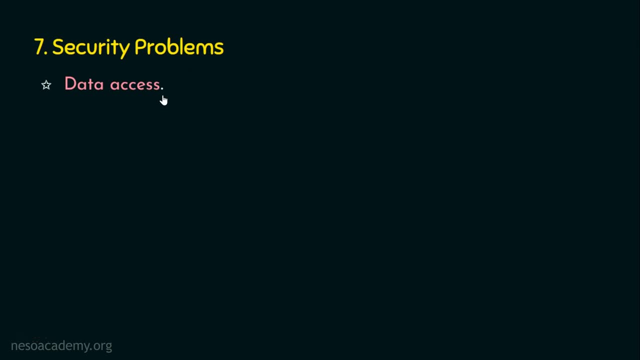 obviously not everyone should be permitted to access the data, so we are required to restrict the data access. so what I mean to say in simple terms is we want to provide authentication as well as authorization, so there are multiple authentication mechanisms so that we can identify whether the right user is. 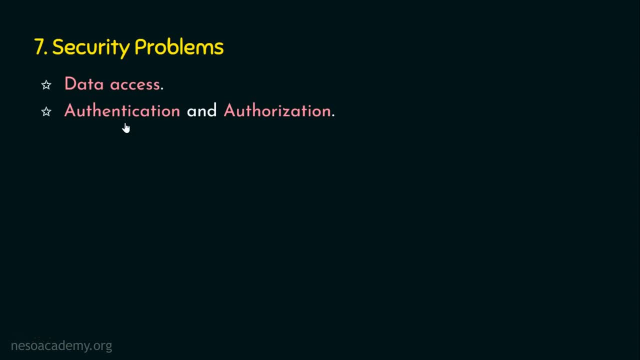 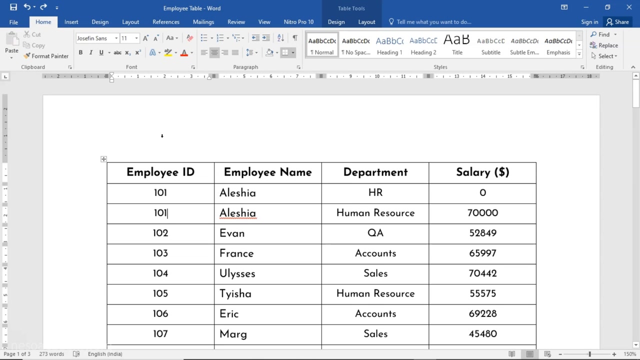 accessing the system or not. so authentication is all about identifying the right person. is accessing the system or not? say, password is one of the two. the authentication mechanisms- biometrics, facial recognition, voice recognition- all these are authentication mechanisms. let's take the file in this file. let's assume we want to restrict access to this file. so what we can do, we 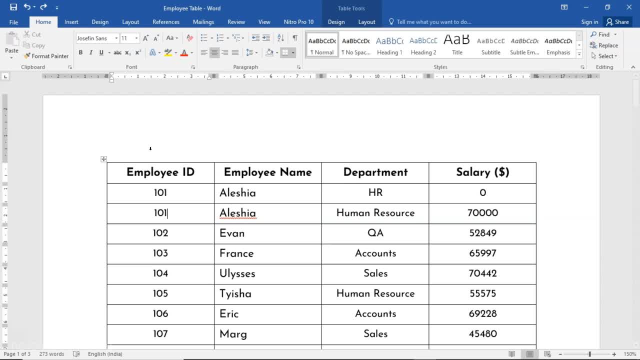 can go to the option security and we can lock this file. so whenever any person opens this file it will ask for the password. so if he gives the right password this file will be opened. otherwise this file will not be opened. let's assume two people have access to this file and both knows the password. 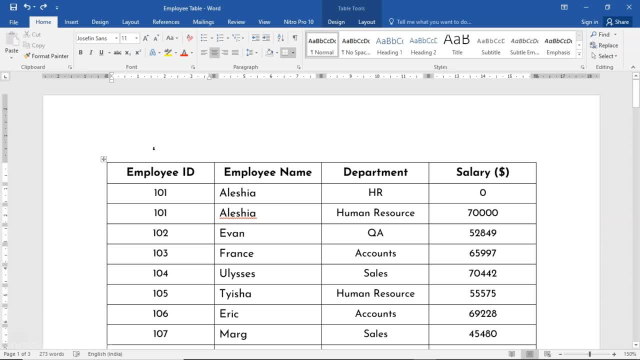 and obviously both will be getting the same privilege. let's name them as A and B. A can see employee ID, employee name, department and salary. similarly, B can also see all these four columns. let's assume B should be restricted from seeing the salary column. in that case, is there any way to lock this particular? 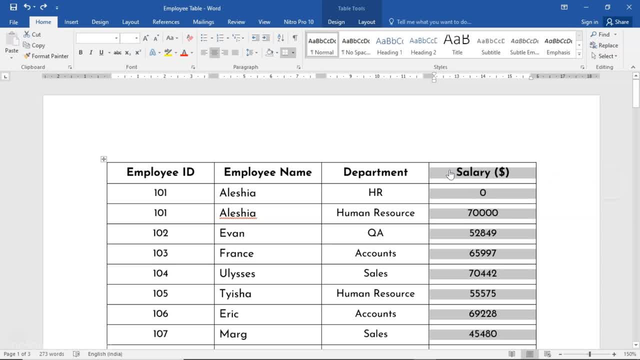 column from B in file system. it's really difficult, isn't it? but in databases we can create multiple views and we can grant the privilege according to the users roles and responsibilities. a normal user will have lesser privilege when compared to database administrator, so database administrator has the complete privilege over the database, but 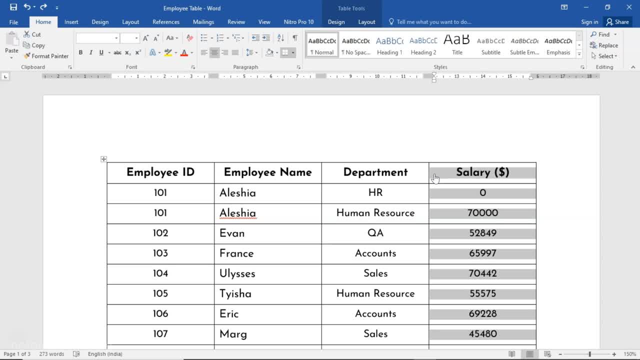 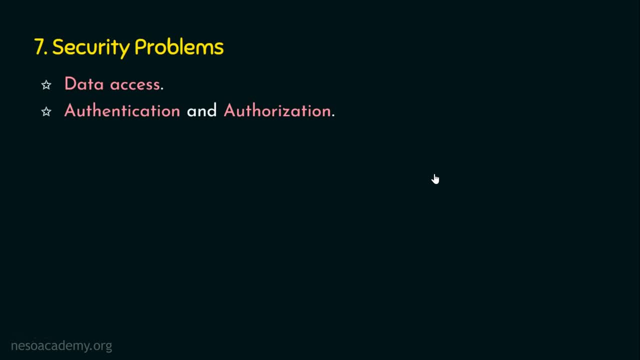 not an end user or an IV user. don't worry about the users. in the coming lectures we are going to see different users of databases, so we will understand things clearly there. so what I mean to say here is we need to have authentication and authorization techniques for the data that is stored. 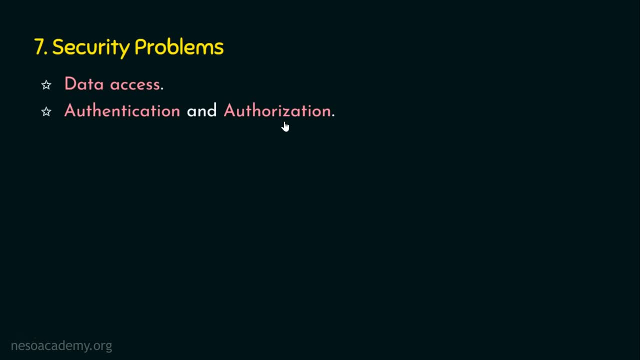 in the file system or in the database system. but the problem is, providing the these things to the file system is really difficult. so databases are really powerful, even addressing security problems. and I'll give you one more example. suppose if we have multiple files in multiple different locations. 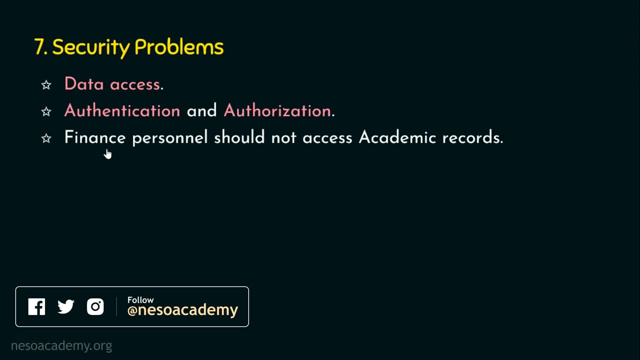 and each file is having different different data. in a university there is a finance personnel and this guy should not access academic records and enforcing this access constraints in file system is really difficult. we understand that finance related data only finance personnel should deal with, but if it is, 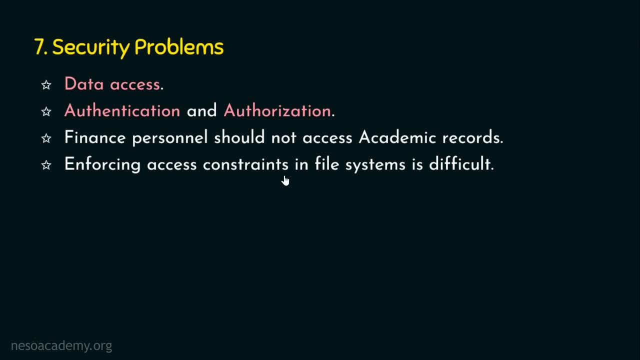 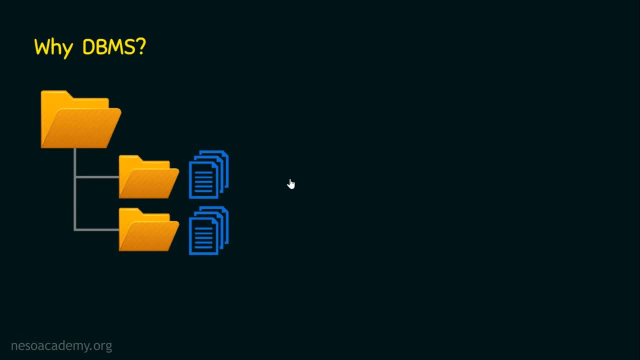 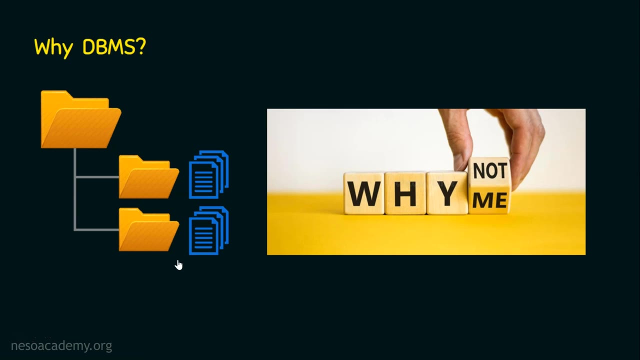 enforcing such access constraints is really difficult. so we have discussed all the seven points in this presentation. I hope now you can understand why do we need database management systems over file systems. because we have seen a lot of drawbacks with the file systems and that's why we wanted to move our 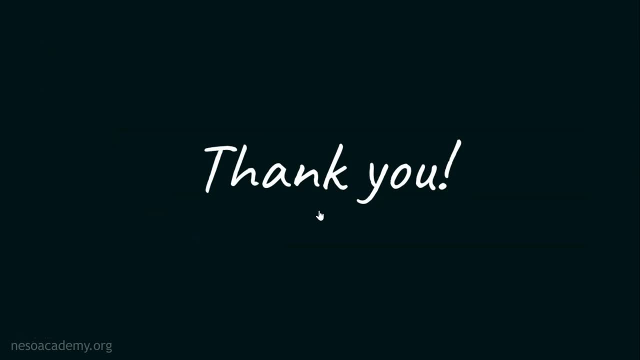 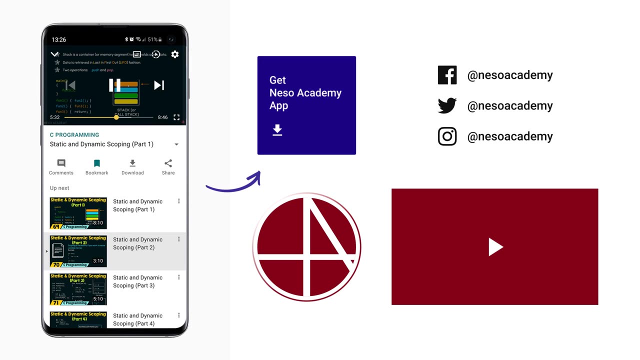 attention towards database management systems. I hope the session is informative and thank you for watching you.